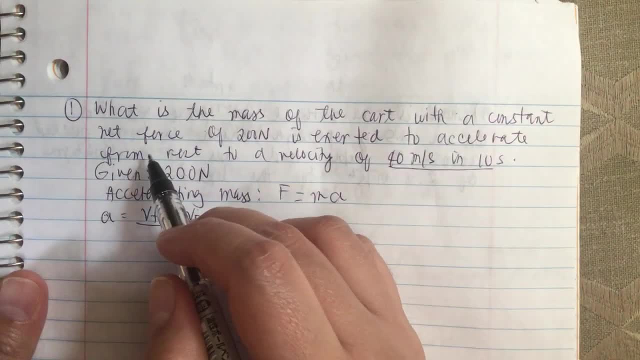 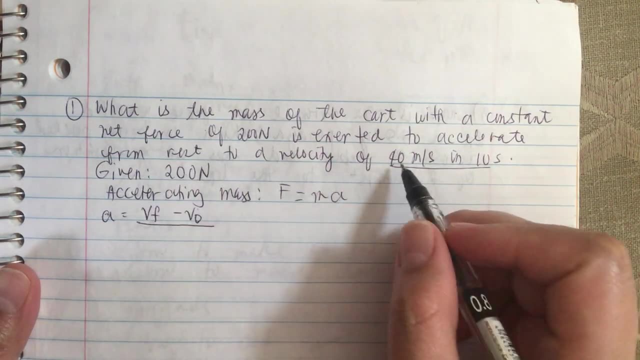 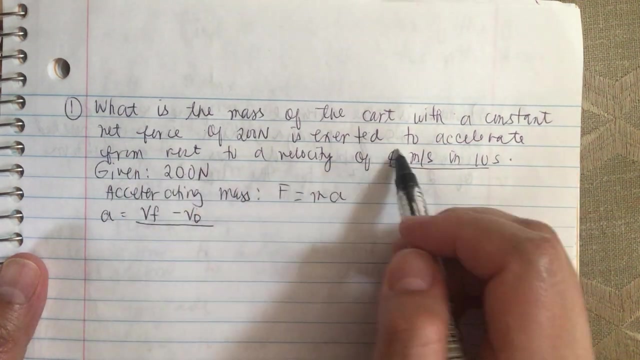 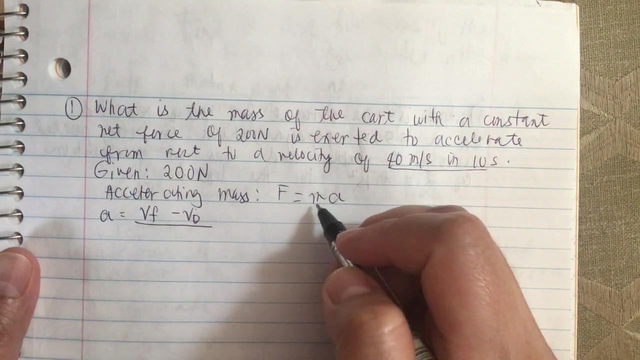 What is the mass of the cart? of a constant net force of 200 newton is exerted to accelerate from rest to a velocity of 40 minutes per second, in 10 seconds Given. so given. so they give us 200 N or newton. the accelerating mass is equal to F, is equal to M times A or mass times the acceleration. 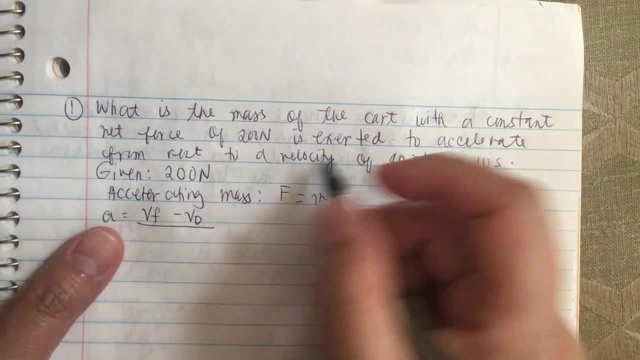 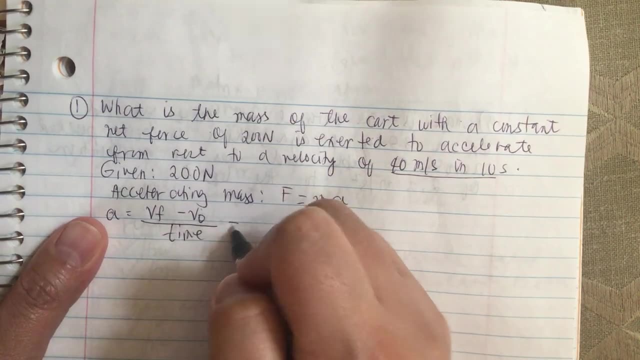 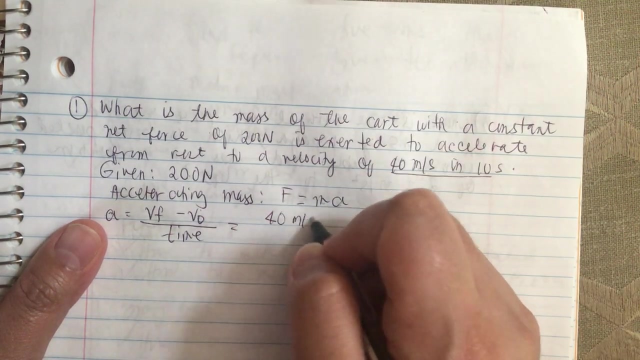 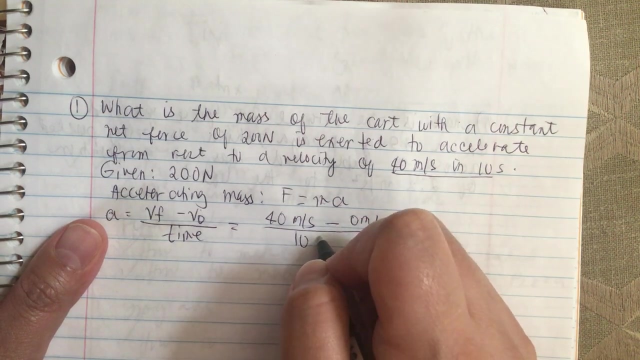 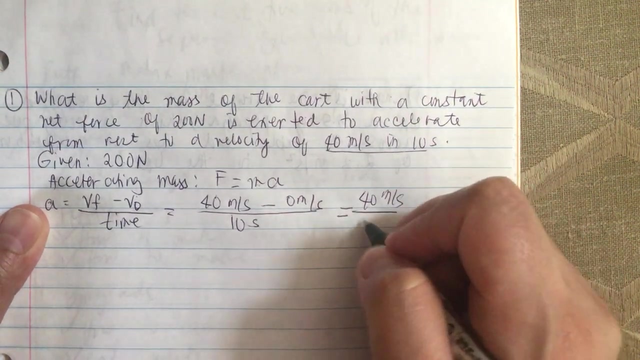 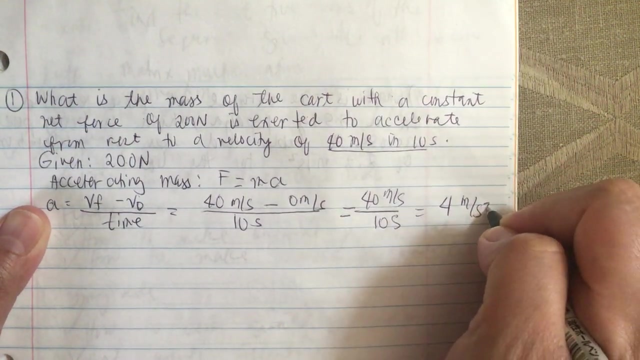 So we have to find A first, so our acceleration, so it's the change in velocity over time. So this is equal to: so 40.. 40 minus 0 over time, which is 10 seconds. So this is equal to 40 over 10, or this is equal to 4 second squared. 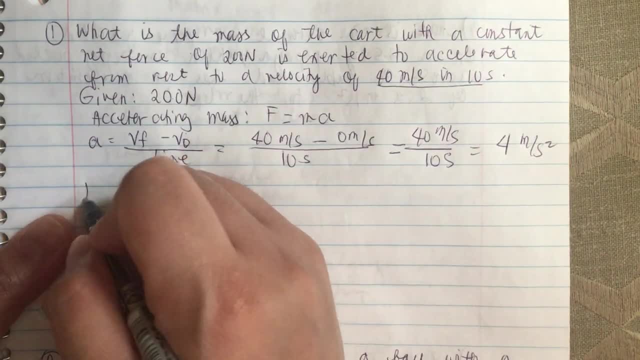 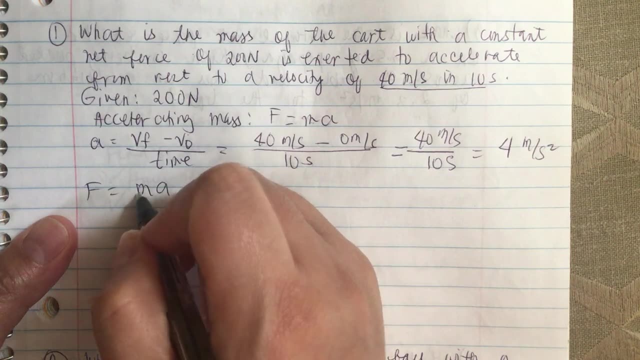 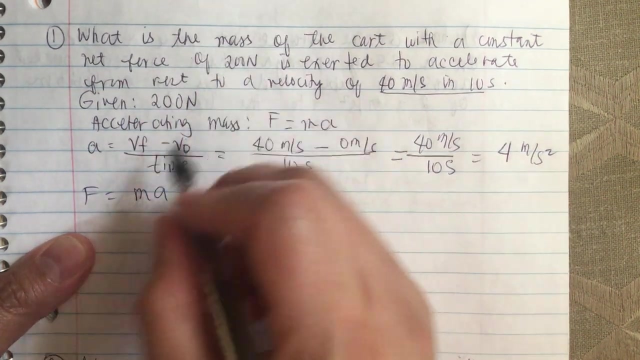 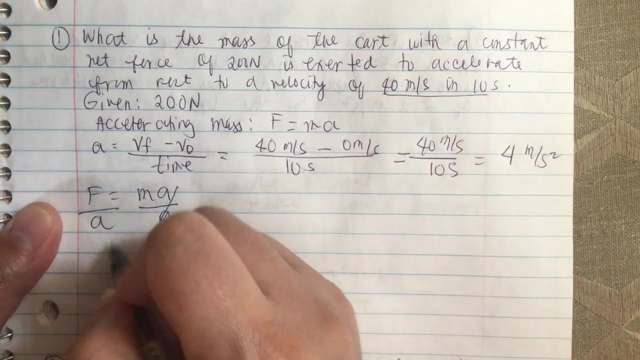 So now we can use this formula now. So F is equal to M times A, or mass times acceleration, or we can rearrange this to the asked for mass, So we subtract A, So we have M is equal to the force over acceleration. 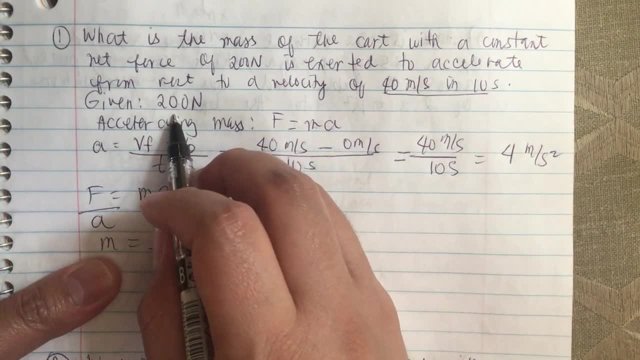 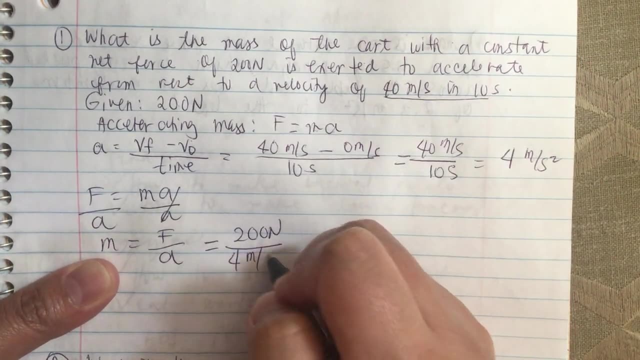 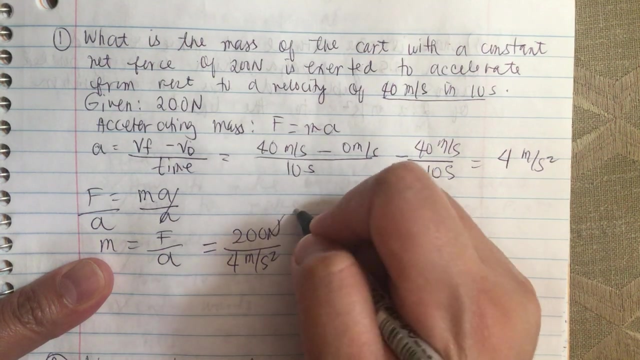 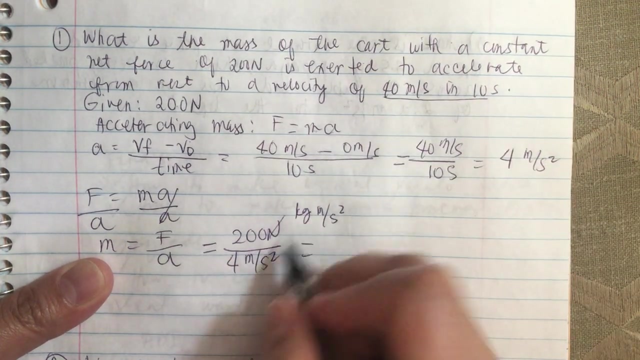 So they give us 200.. So this is 200 newton over a. we find a. so this is equal to. so one newton is the same as um. this is kilogram and per second squared, So we just change the units. 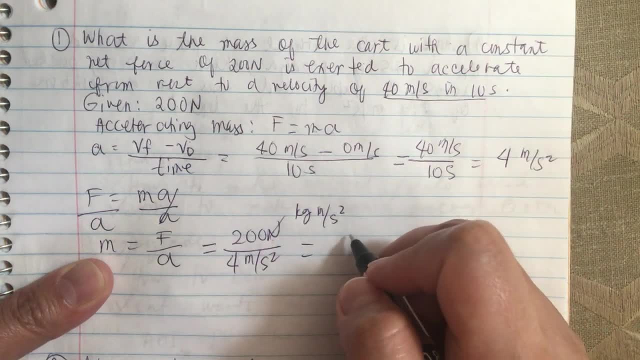 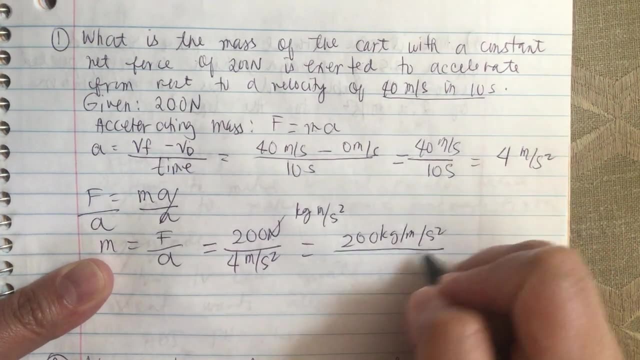 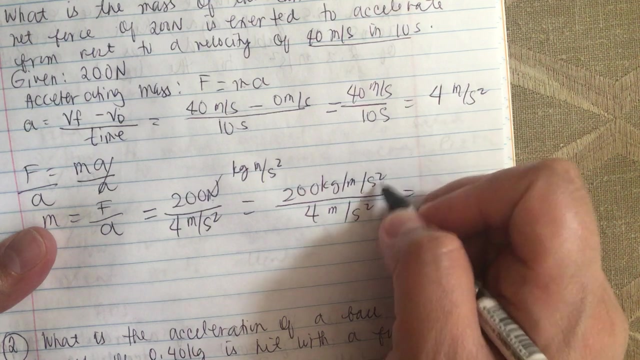 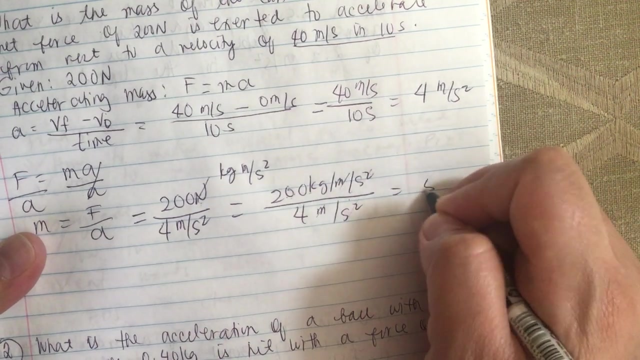 This is: these are the same. So this is equal to 200 kilogram M Um per second. so for um per second squared. so now they have the same unit. So this one cancels that one. So we have 200 kilogram. 200 divide four is equal to 50 and we just have the kilogram left. 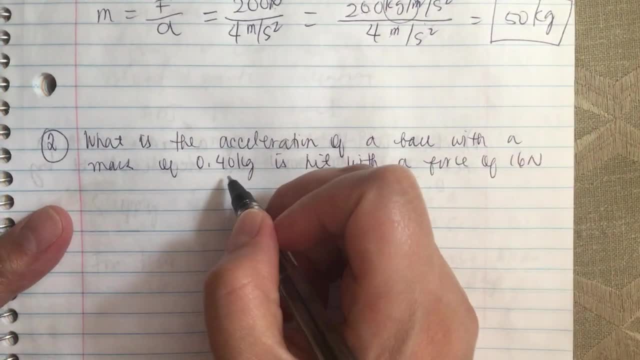 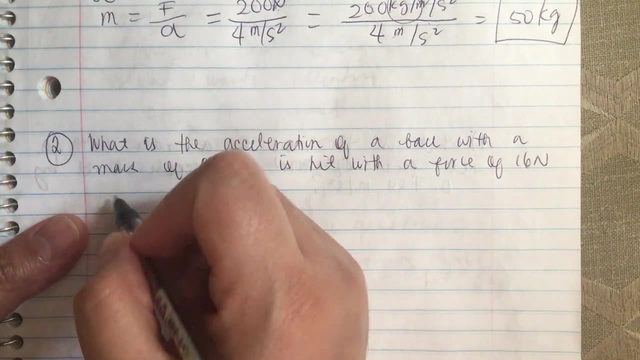 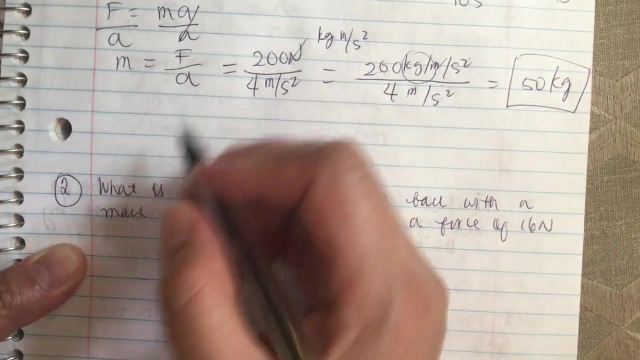 So what is the acceleration of a ball with a mass of point 40 kilogram is hit with a force of 16, um Newton. So we use the same formula. so the asked for acceleration, So we solve for a and a is equal to F over M. 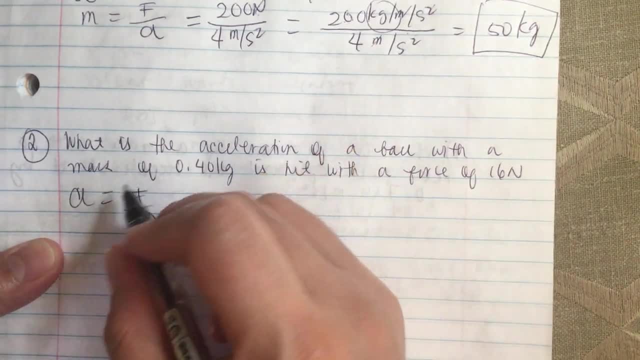 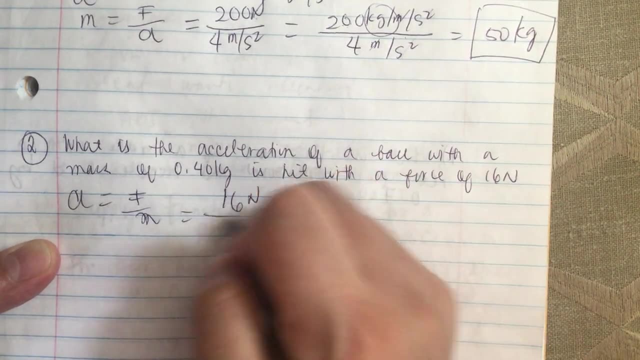 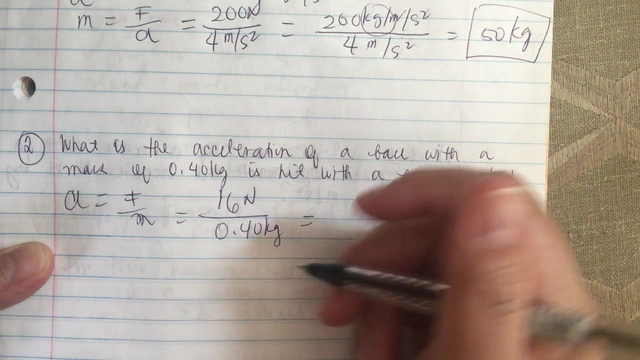 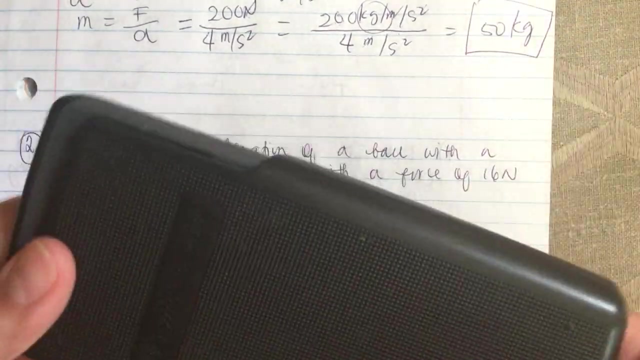 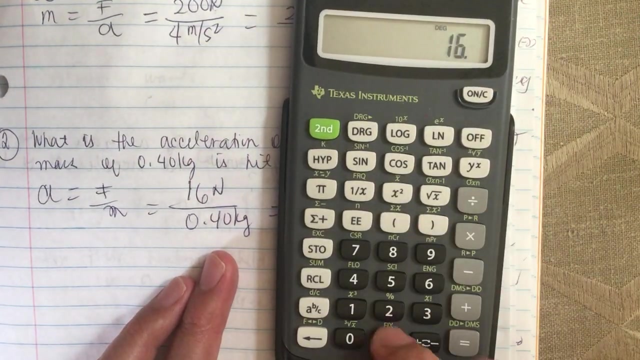 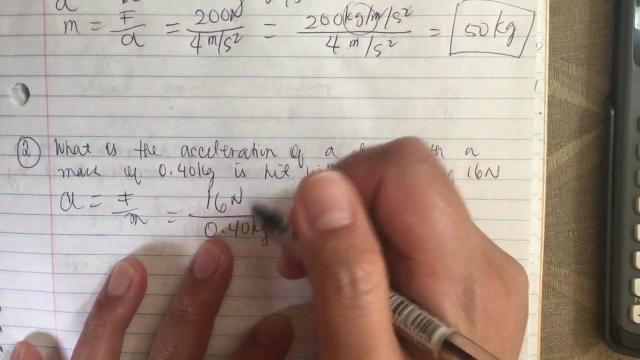 So just rearrange it. So they give us F, so 16.. Okay, Over M, they give us M, So 16 divide 40 is 40. It's equal to 40. So now one Newton is the same as um one kilogram. 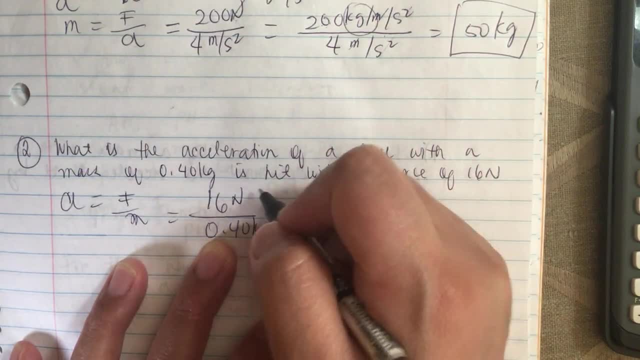 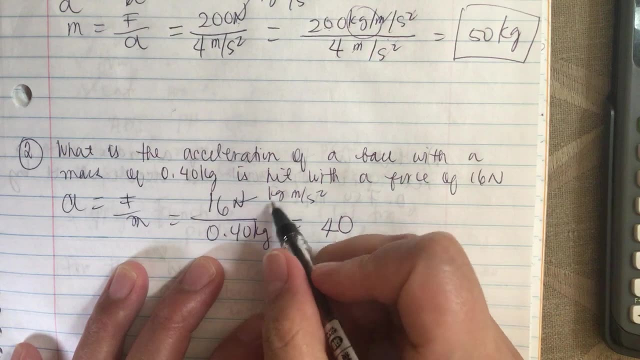 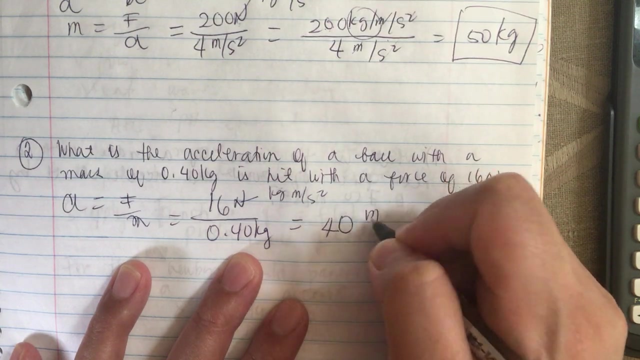 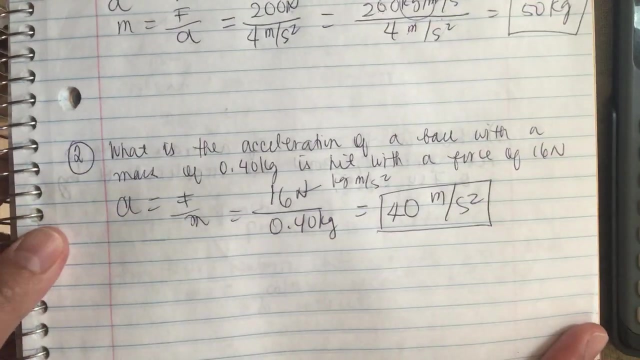 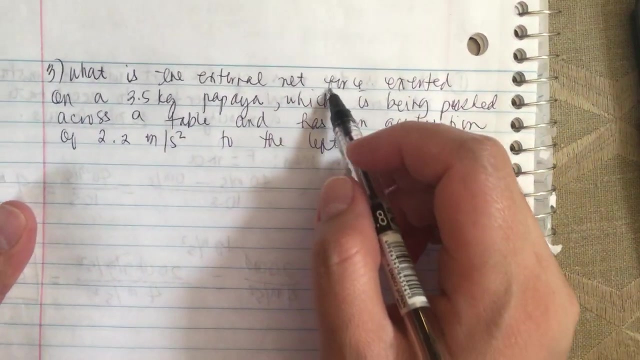 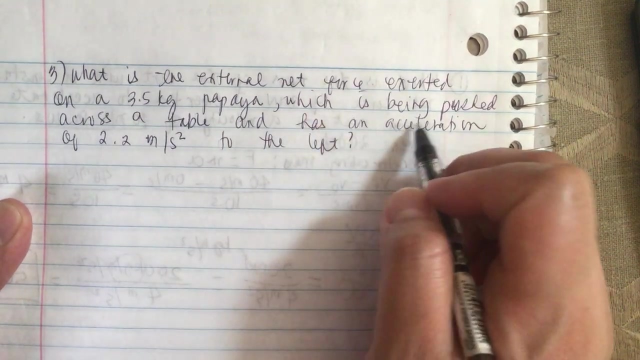 ms squared. so let's change this unit to kilogram, ms squared. so now it cancels the kg or kilogram, so we have 40 m over s squared. what is the external net force exerted on a 3.5 kg papaya? kilogram papaya which is being 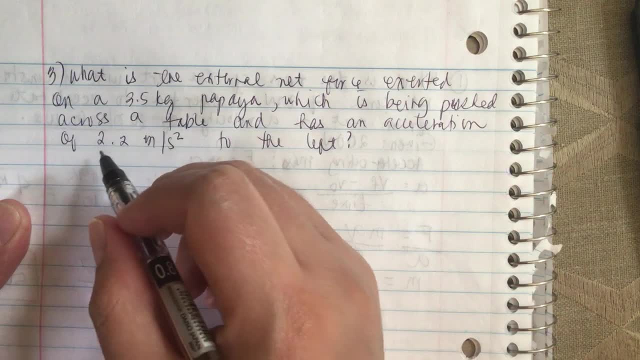 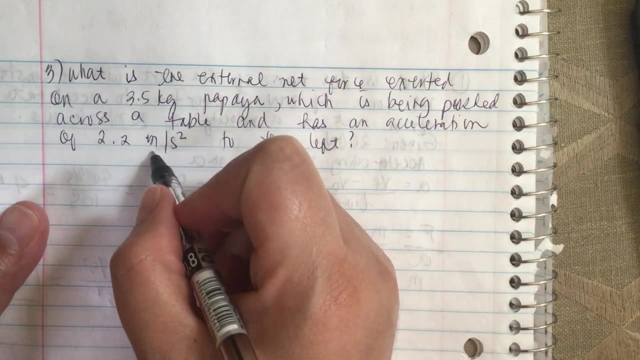 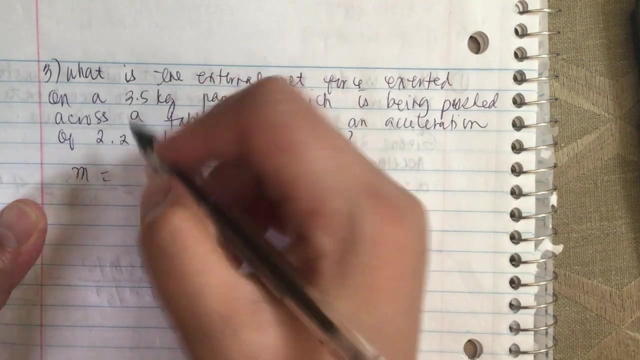 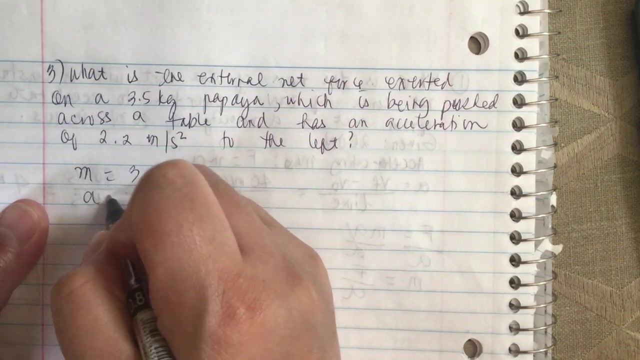 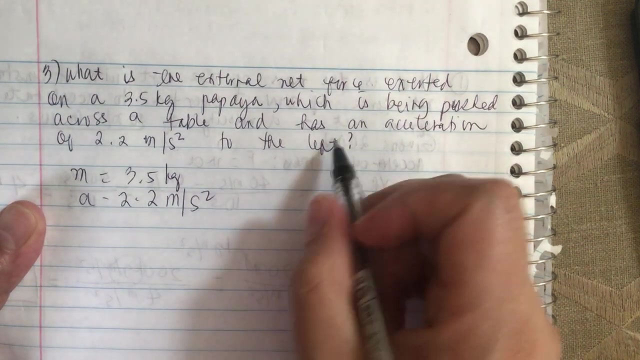 pushed across the table and has an acceleration of 2.2 ms squared to the left. so so, so, so, so m. so they give us the mass, which is 3.5, and they give us a or the acceleration, 2.2 m per second squared. 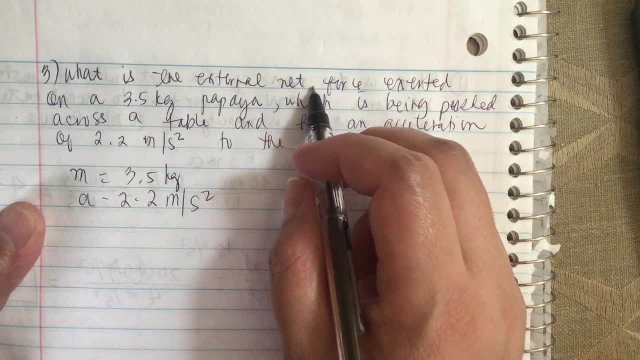 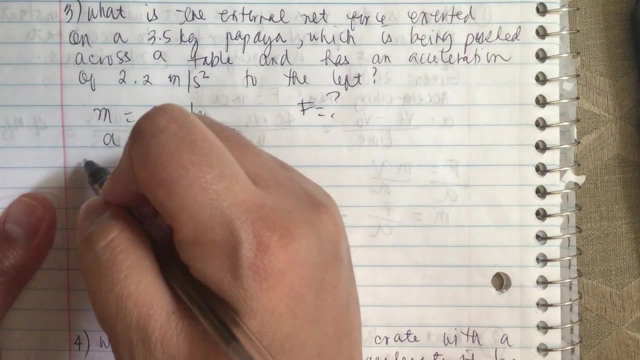 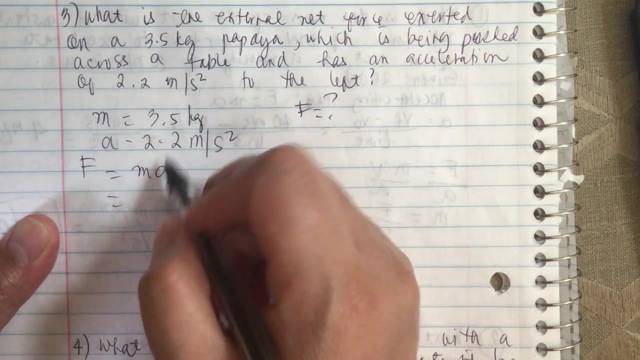 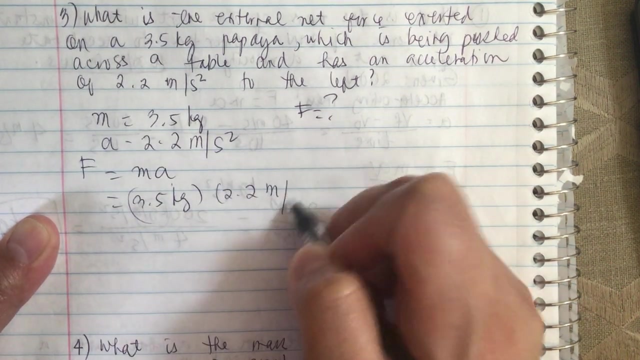 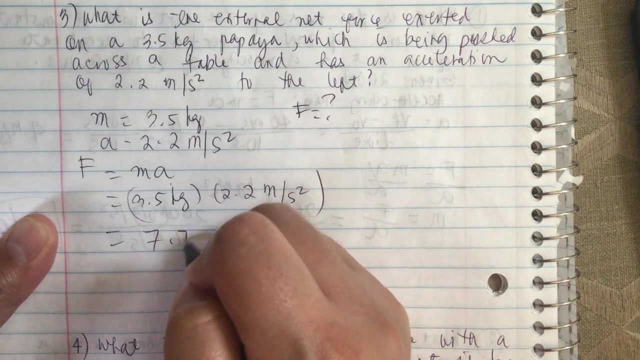 and they asked us the um f, the net force, force. so we use this same formula: f is equal to m times a, so m is equal to 3.5 kilogram times a, which is 2.2 m per second squared. so this is equal to 3.5 times 2.2 is 7.7, now the units it's going to be.